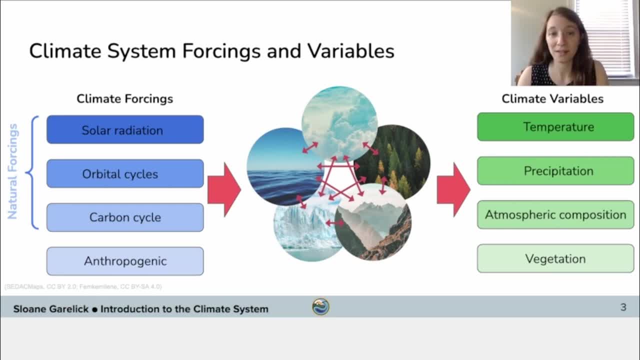 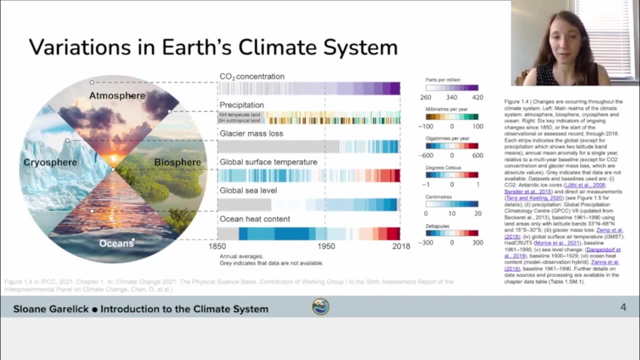 However, today, changes in the climate system are occurring at a much faster rate than the past in response to anthropogenic causes in greenhouse gas emissions. This figure is from the IPCC report and shows changes in multiple climate variables since 1850, and this really highlights the impact of anthropogenic forcings on the climate system. 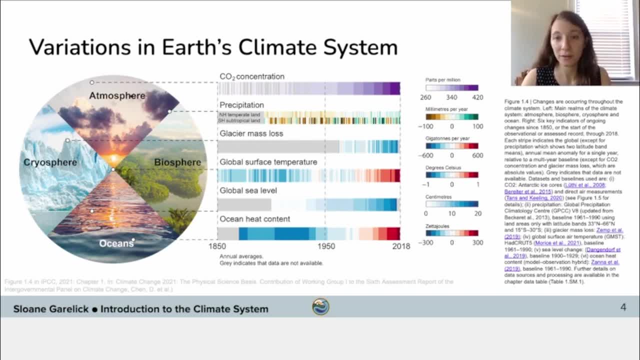 For example, over this time there has been an increase in atmospheric process in the climate system, atmospheric CO2 concentration, increased variability in precipitation, increased glacial mass loss, a warming of global surface temperature, a global sea level rise and an increase in the 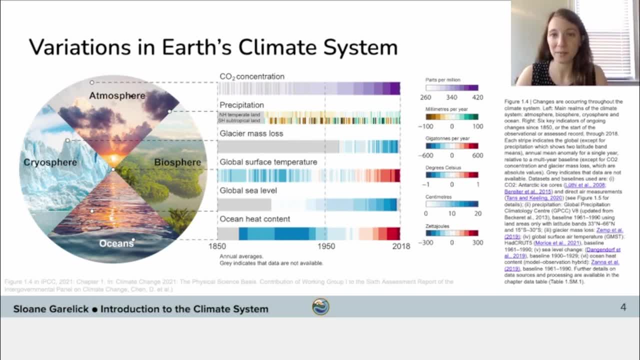 ocean heat content, And these are just a few examples of ways in which anthropogenic forcings have influenced recent climate. Other examples include sea ice loss at the polar regions and terrestrial habitat loss due to deforestation and land use. During the remaining videos today: 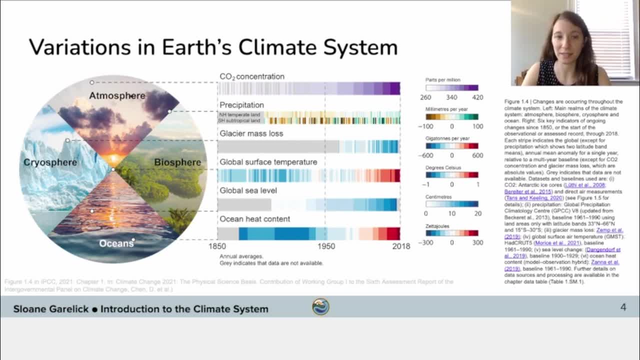 we'll learn more about different forcings and processes of the climate system and how they vary on different time scales. And throughout these tutorials, we'll learn how to use a Python package called X-Array, which is specifically designed to analyze large climate data sets. 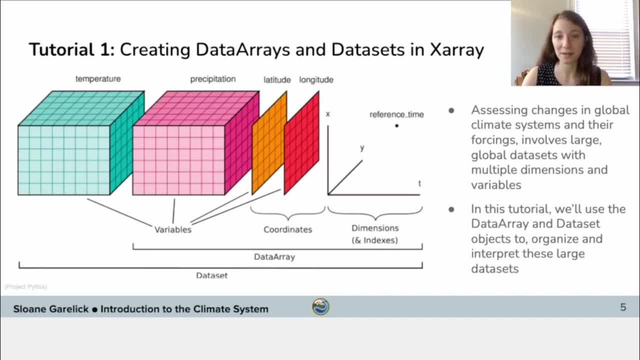 X-Array is an open source project and Python package that makes working with labeled multi-dimensional arrays simple. X-Array introduces labels in the form of dimensions, coordinates and attributes on top of raw data array, similar to those produced in NumPy. X-Array includes a large number 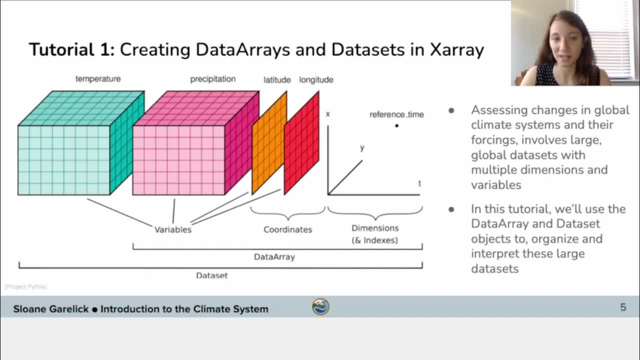 of functions for advanced analytics and visualization of these data structures. Throughout the tutorials today, we'll learn the basics of X-Array and apply some of these tools to the climate data sets to further explore the climate system concepts that we discussed in the videos. 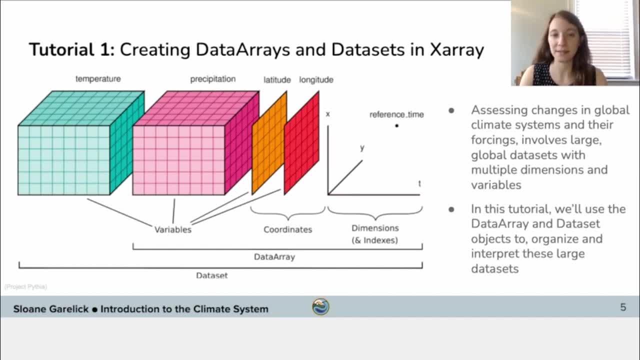 In this tutorial, we'll learn how to create data arrays. that can be used to create data arrays and data sets in X-Array, And both of these objects are used to represent and manipulate spatial data. The data array is one of the basic building blocks of X-Array. In a data array, coordinate names and values. 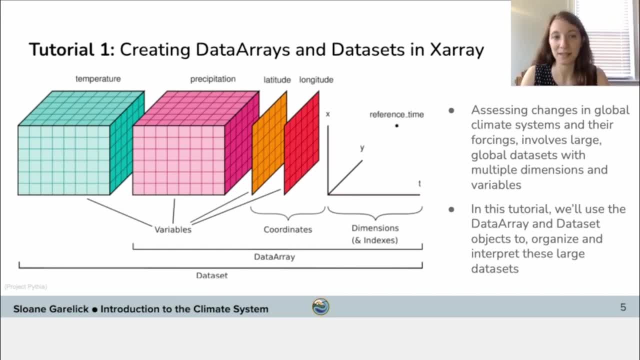 are stored with the data, making it simpler to slice and index the data. Along with the data arrays, the other key object type in X-Array is the data set. This is a dictionary-like container that holds one or more data arrays and can share coordinates.